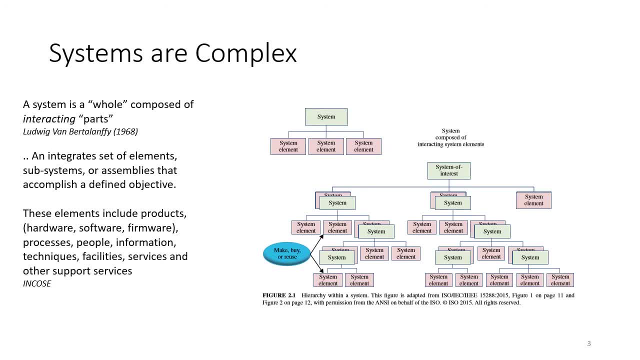 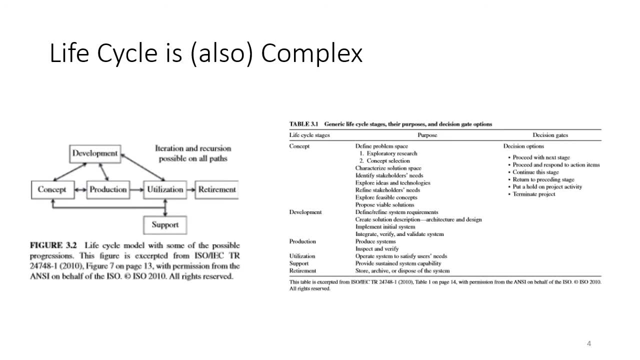 a static interaction but a dynamic interaction, And it's that interaction that creates complexity. So these systems, these systems operate in a life cycle. They're conceived in the beginning, in what's called the conceptual phase, They go through development and end up in production and utilization. And 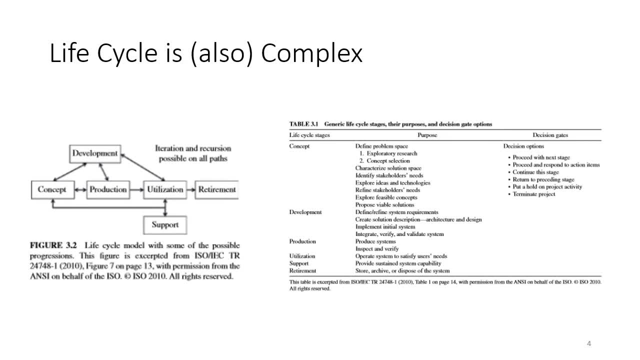 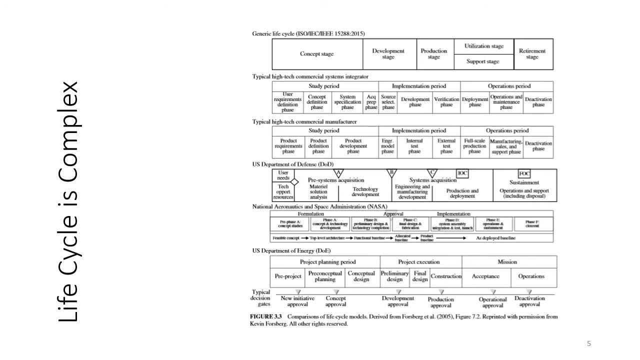 then subsequently these systems are retired. There are a large number of ways of thinking about the life cycle, depending on the kind of system that's being developed. This is figure 3-3 from the system engineering handbook and it's kind of a running list of all. 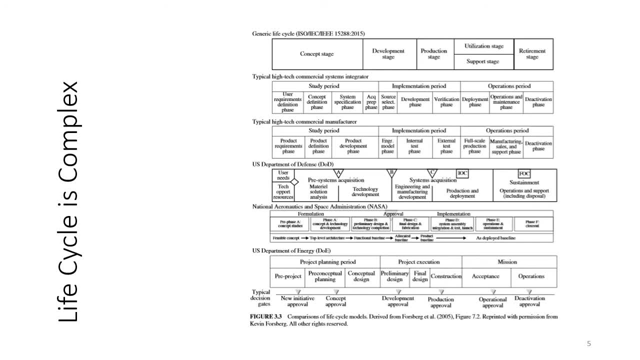 the different life cycles that are used by the Department of Defense, by NASA, the Department of Energy. Those are the three life cycles at the bottom And then on the top is the second one is the high-tech commercial systems integrator and the high-tech commercial manufacturer. 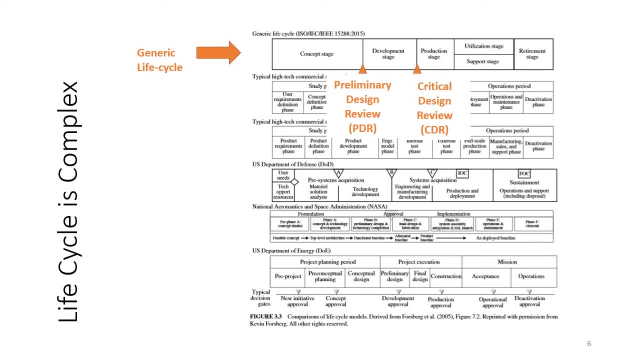 All of these processes. these can be summarized by the generic life cycle process as defined by ISO and IEEE, And there are six stages of that. So the first stage is the concept stage, where the system is conceived and initially scoped out. The second stage is the development stage That's followed. 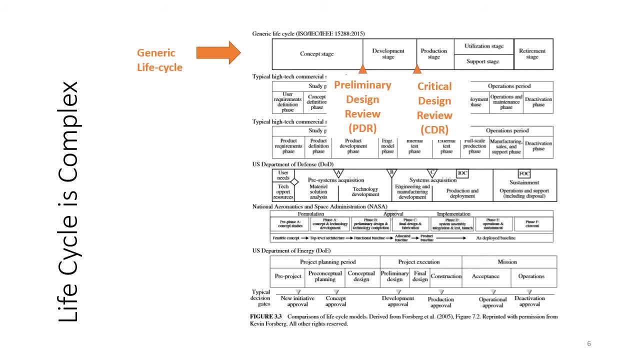 by the production stage, where the system is built and produced, manufactured, and then it goes into utilization, that is supported by the support stage, no pun intended, And then, finally, the system goes into a retirement stage. So the six stages: concept, development, production, utilization, support and retirement. 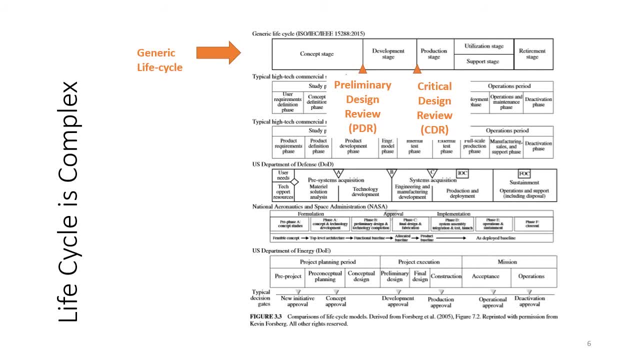 And, of course, the system engineers. we are responsible for managing this complete life cycle. Two of the most critical tasks that system engineers are responsible for is something called the preliminary design review, And that is a gate, a checkpoint, to go from the concept stage to the development stage. 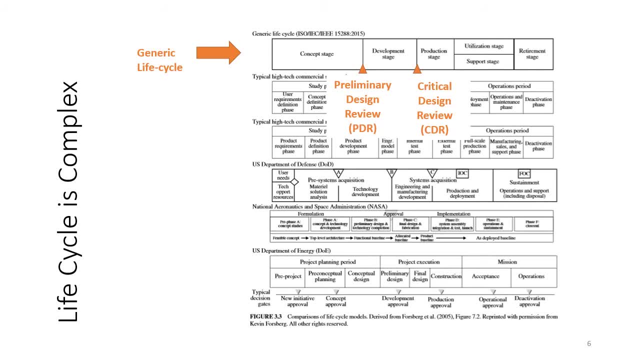 So the system engineers would coordinate amongst all the suppliers and all the components and developers of the components and make sure that we have a system that will meet the needs and that we can build it on time, on cost and with the required quality. So once the project is approved, then the next stage is to go into the development stage. 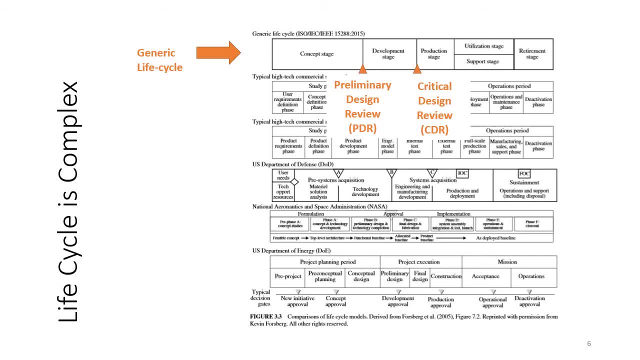 And that's the actual process of doing the hard engineering work to come up with a manufacturer-world product. At the end of that stage there's something called a critical design review that takes place, And that's to make sure that, before we go into production, that we've crossed all the T's, dotted all the I's and we have a good system design. 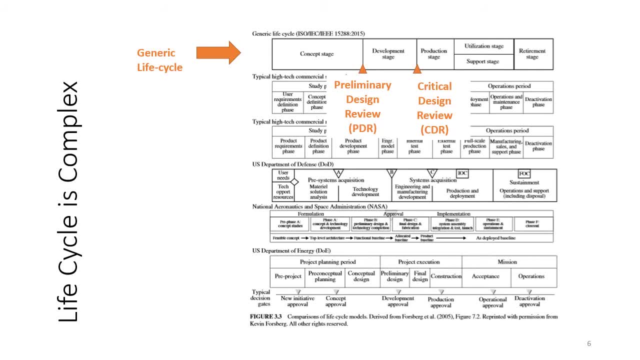 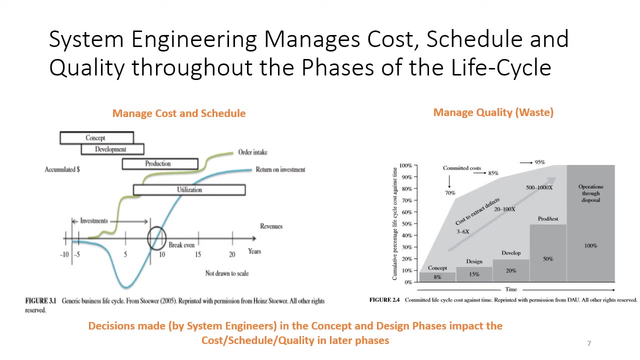 So that's the process. So that's the process. Of course there are lots of variations of all of this, but that's the generic life cycle and the two key responsibilities of system engineers. So the system engineering kind of sits at this nexus of quality and the performance of the system. 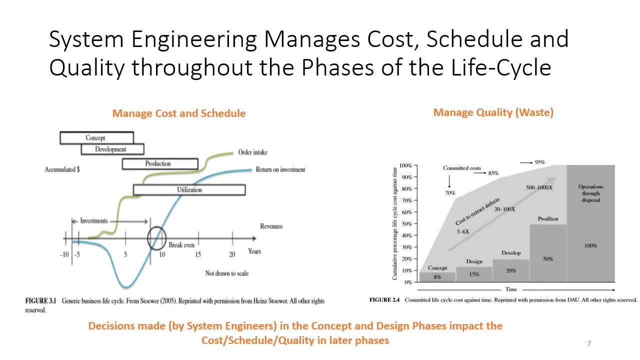 but also managing the cost and schedule for development, And so the Nkosi handbook has These two diagrams. the one on the left kind of emphasizes the point that the system engineers have to manage the cost and the schedule throughout the life cycle. 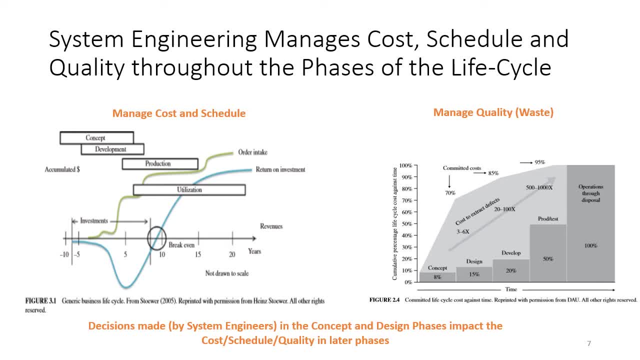 And then the figure on the right-hand side points out that the work that's done in the initial phases- the concept and the design phase- have big impacts in the later phase. So it is a lot cheaper to identify a bug in the early phase. 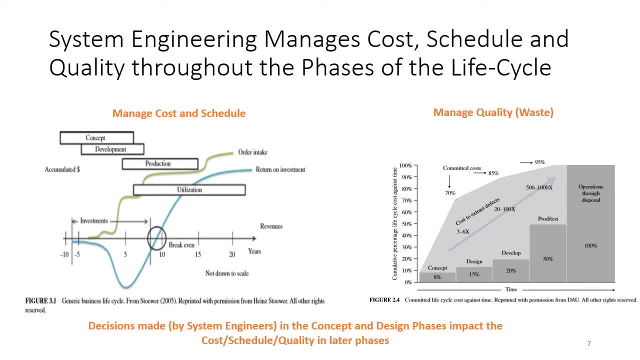 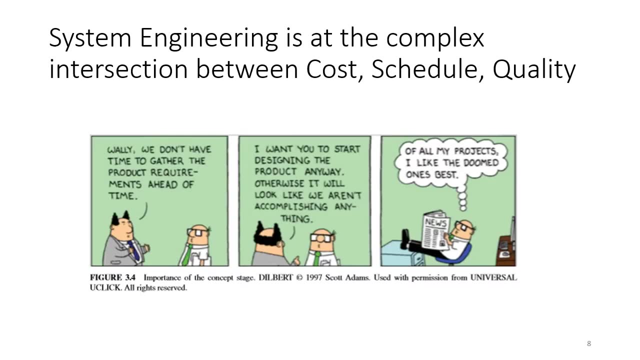 than it is to identify and fix a bug that's in production, for example. So the system engineers have to kind of manage this quality-cost schedule and that's an important responsibility that they have. So to kind of emphasize that point, figure 3-4 in the system engineering handbook has our favorite cartoon, Dilbert. 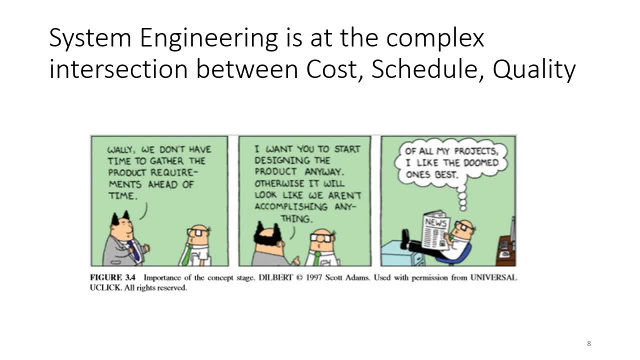 And in this cartoon you kind of get the sense for the issues of not only managing the requirements and the design of the system, but also the staffing and the development process. And in this case the pointy-haired manager says: Wally, we don't have time to gather the product requirements ahead of time. 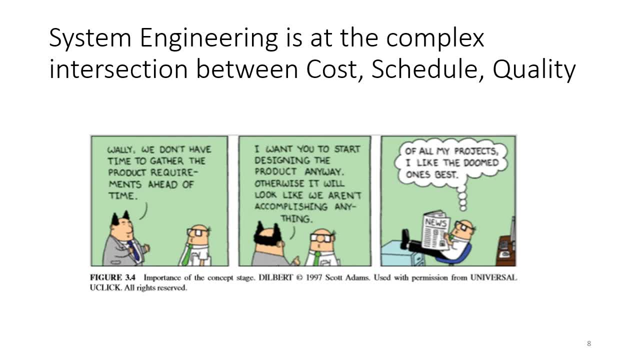 I want you to start designing the product anyway, Otherwise it will look like we are not accomplishing anything. And of course, Wally says. Wally goes back to his desk, he pulls out a newspaper. I guess he would really pull out his cell phone nowadays and he would be reading the news, catching up on social media. 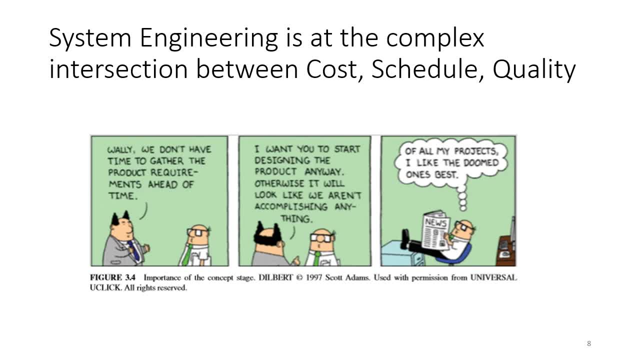 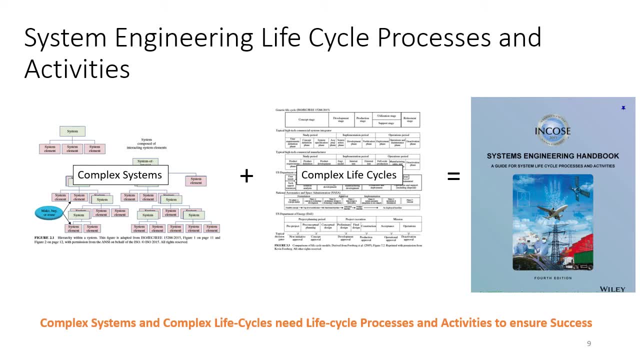 And he thinks to himself: of all my projects, I like the doomed ones the best. So we've got these complex systems that we've talked about, with lots of components, non-homogeneous components and interaction between the components, And then we have these complex lines. 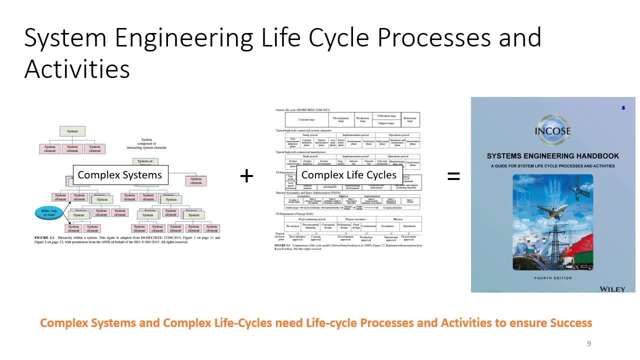 These life cycles with at least six stages- concept, development, production, utilization, support and retirement- And you put those two things together and you can't just do it ad hoc. It has to be a more structured thought-out process. 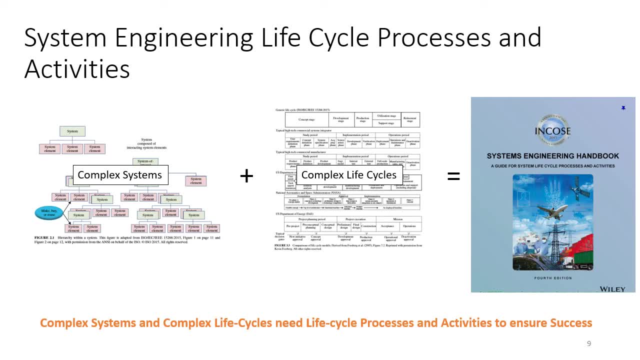 So, thanks to the hardworking Nkosi system engineers, they've put together the System Engineering Handbook to serve as a guideline for defining the life cycle, processes and activities that will ensure that the system is functioning, And I think that's the key to our success in these complex systems with complex life cycles. 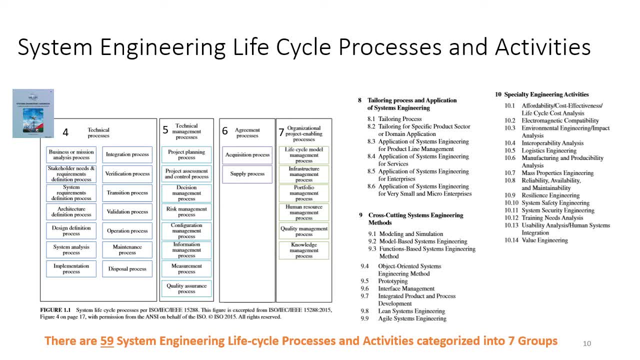 So the handbook is this massive document, And let me tell you right off the bat, as you can see in the orange text on the bottom, that there are a total of 59 system engineering life cycle processes and activities that are identified in the handbook. 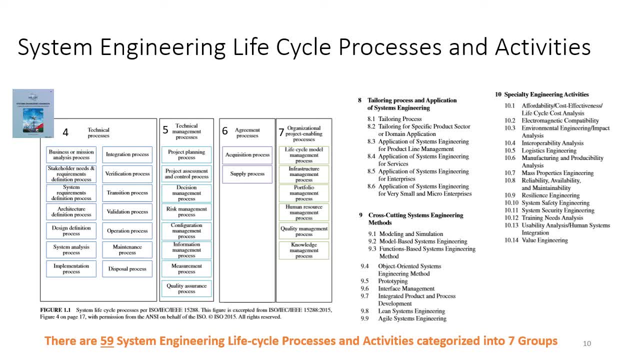 Those processes and activities are organized into seven groups. So let's go through those seven groups and just do a quick overview of the processes and activities, And of course, the remaining videos in the series are going to describe each one of them in more detail. 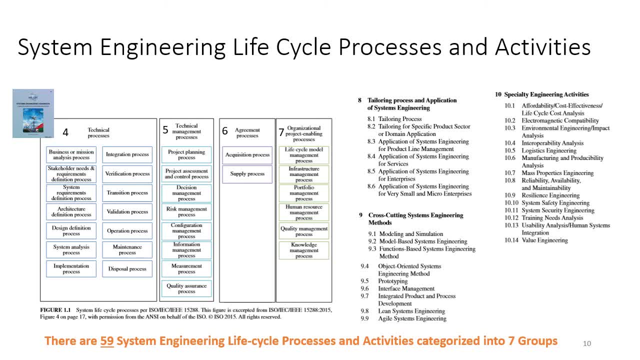 So, starting on the left-hand side, we have the technical processes, And those are all the things that you would expect engineers and system engineers to do, from establishing the business or mission of the system, Evaluating the stakeholder needs and developing requirements, coming up with the architecture, designing, performing system analysis, implementing. 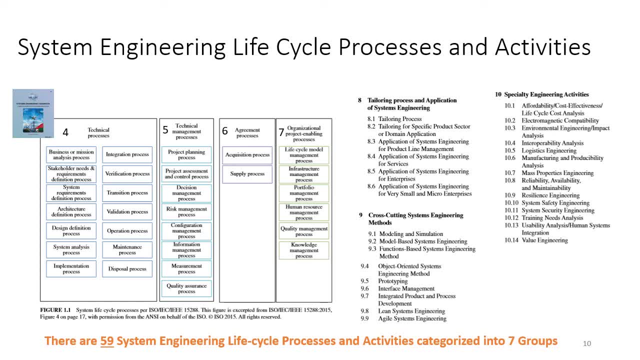 And then, once the pieces are starting to the components are developed and implemented, you go down the backside of the V with integrating them and then performing all of the testing before fielding, maintaining and then finally disposing of the system. So those are all the things that you would expect engineers and system engineers to do, from establishing the business or mission of the system. 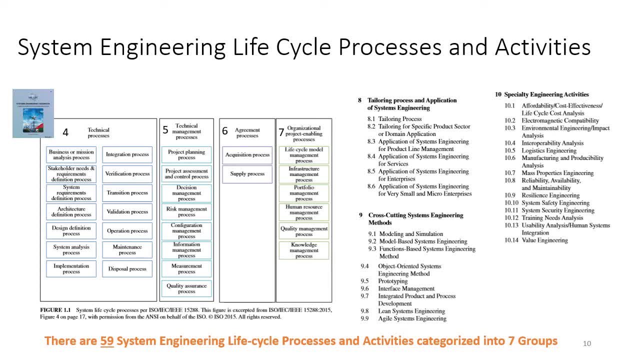 And those are all the things that are clumped together in that technical process group. Chapter five has the technical management processes And of course all of that is associated with developing a project plan and managing the project. Chapter six is the agreement process. 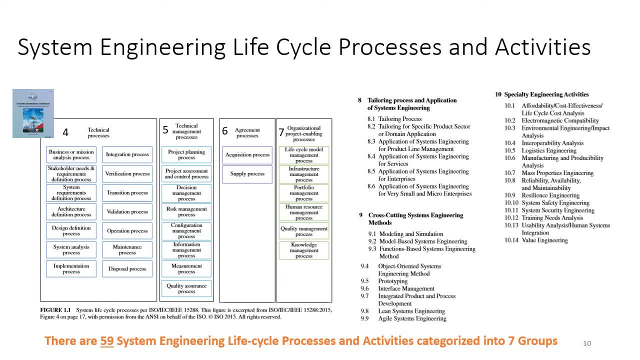 And that's the contractual support for purchasing all of the services that are needed to do the development, as well as the components that will be needed for manufacturing, production and support. Chapter seven has some organizational project enabling processes. I think of these as kind of meta processes that allow one to manage the workforce that's performing the technical management and agreement processes. 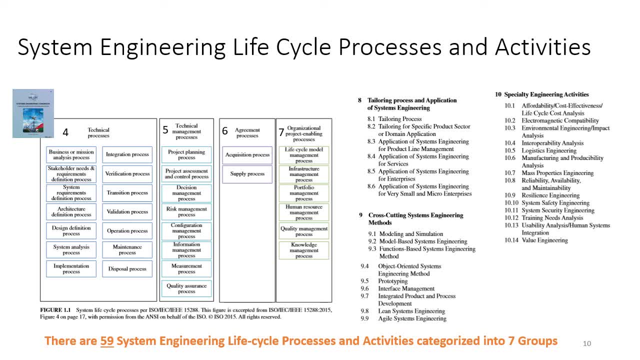 So these are things that override the whole lifecycle and ensure success. So these are things that override the whole lifecycle and ensure success. So these are things that override the whole lifecycle and ensure success. And then, on the right hand side, and chapter eight, nine and 10, are these cross cutting processes? 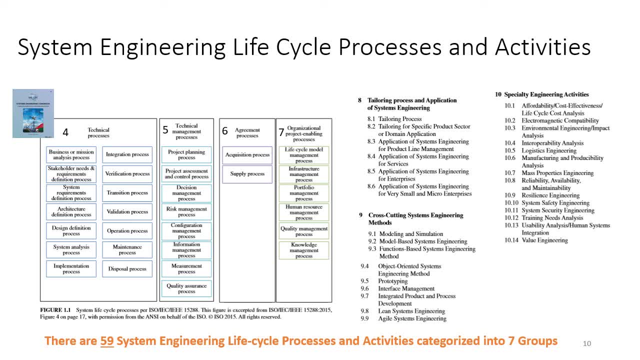 So these are things that are used throughout: the technical processes in Chapter four, the management processes in Chapter five To a lesser extent the agreement processes in six and the organizational project enabling processes in seven, So for example in Chapter ten. 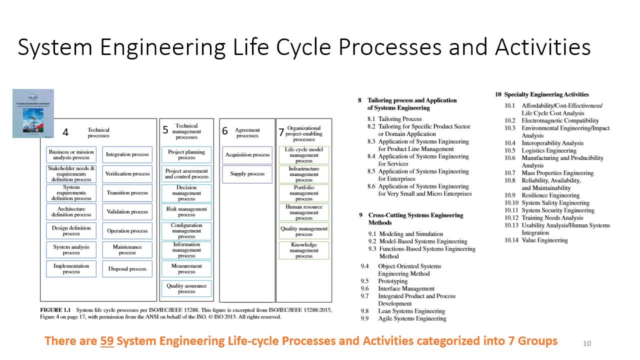 There is chapter 10.8 discusses reliability, availability and maintainability and of course, those are things that need to be defined early in the requirements. They need to be achieved through the design of the system and they need to be tested in the verification and validation testing phases. 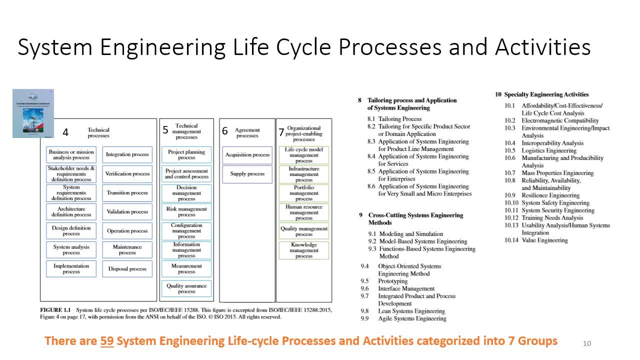 The same thing is true for 10.10,, which is safety engineering, and of course 10.13,, the usability design, making sure that the system that's defined by the requirements early on has the characteristics of sound user interfaces, and then checking and testing those user interfaces throughout the remaining of the process. 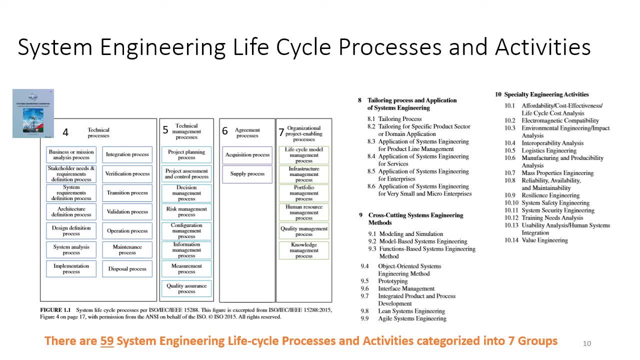 So that's an overview of the system engineering handbook 59 system engineering life cycles, processes and activities and they're organized into seven groups And, of course, in this video series we're going to make learning those 59 and knowing which groups they fall into a fun, entertaining activity. 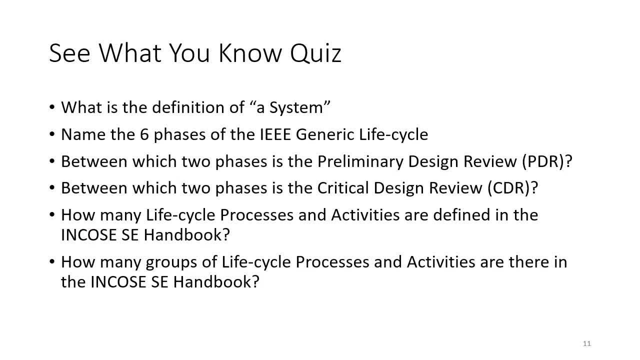 Right. So let's see. let's see what you know. This is a good time for you to grab a pencil and paper, put the video in pause and see if you can answer these questions. So what is the definition of a system? 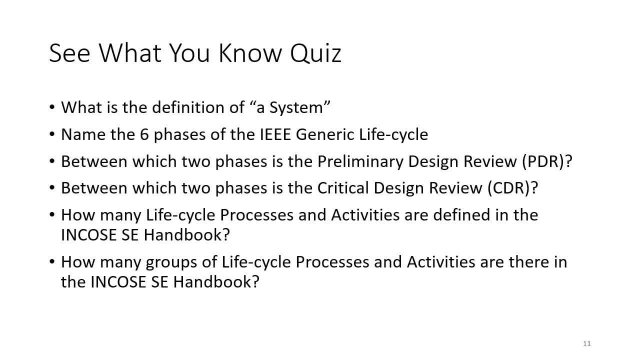 What is the six phases of the IEEE generic life cycle? Between which two phases is the PDR? Between which two phases is the CDR? How many life cycle processes and activities are there in the handbook and how many groups? So please hit the pause button here and see if you can jump in. 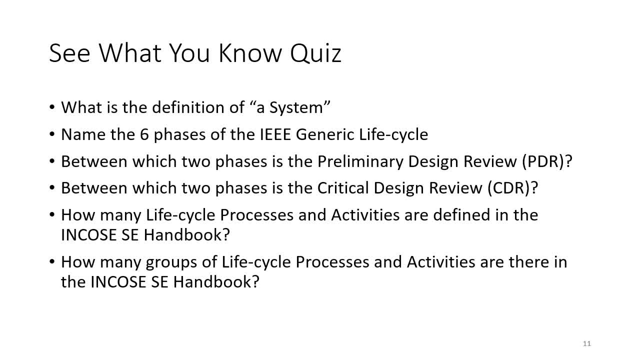 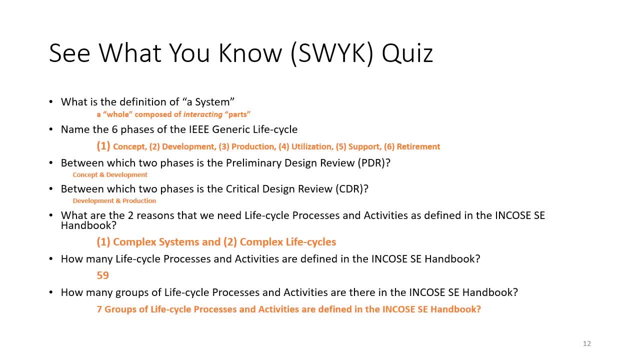 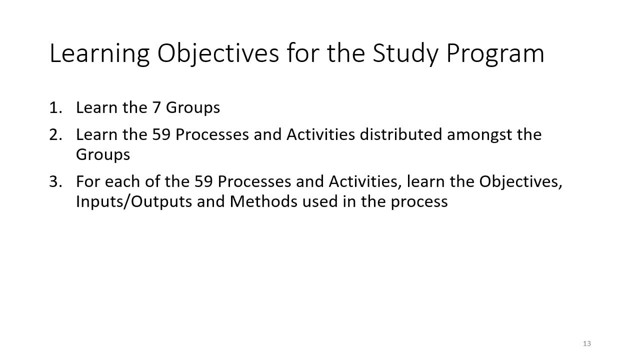 And see if you can jot down the answers to those questions, And when you're ready you can hit play. And here are the answers. Feel free to check yourself. So the remaining videos are going. you're going to learn the seven groups of processes and activities. 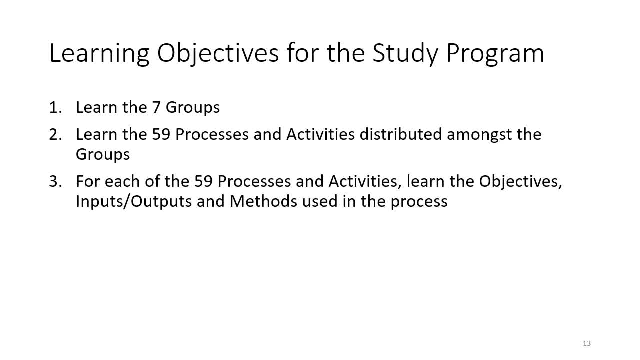 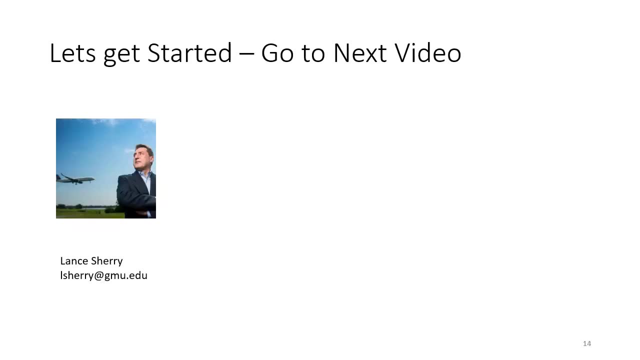 You're going to learn all 59 processes activities And for each process activity you're going to learn the objectives, the inputs, outputs and the methods that are used in that process. So congratulations for getting started and look forward to the journey together. Go system engineering.